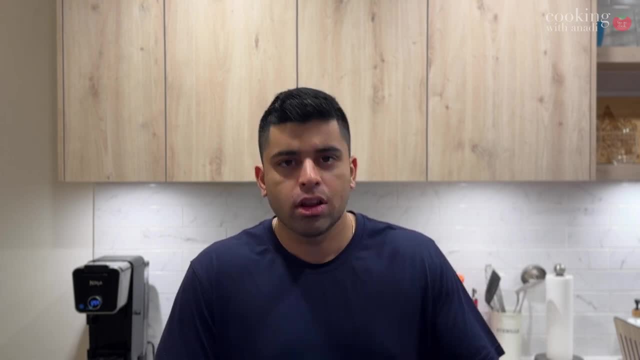 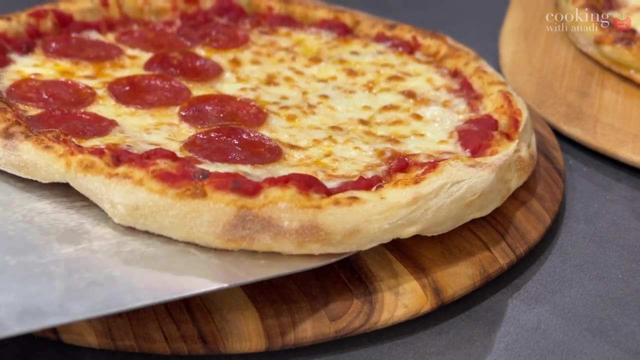 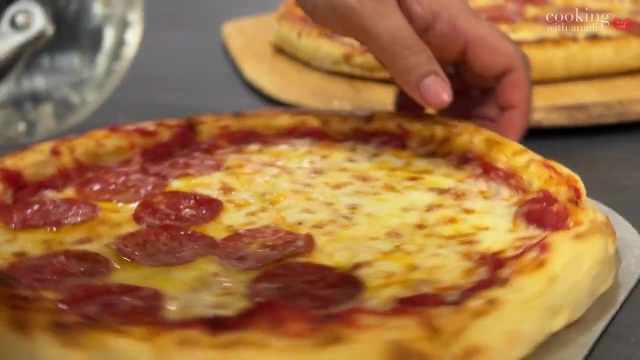 And then people started asking me about: hey, so what are the differences between bread flour and the double O flour? Well, here it is. And when it comes to pizzas made with these two types of flour, well, take a look here. Can you tell just by looking which one is which? Well, you're gonna have to stay. 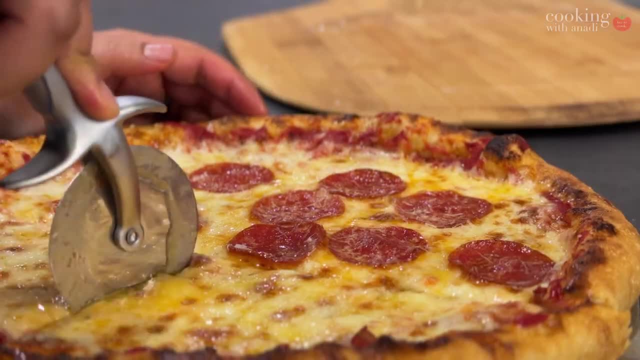 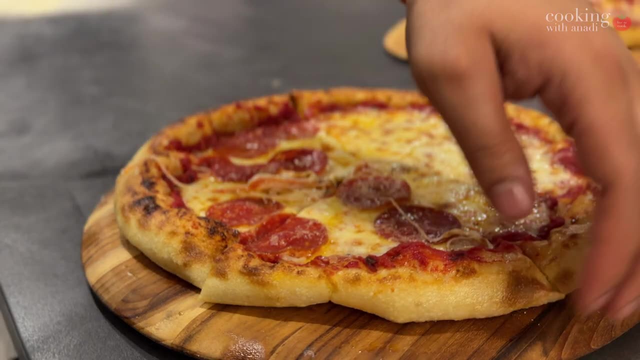 tuned until towards the end of the video to figure out, well, which one is made from double O versus bread, Because they are very different. So I'm gonna start with the bread: flour and the double O: very similar. well, that's what we have this video for: to really see what sets. 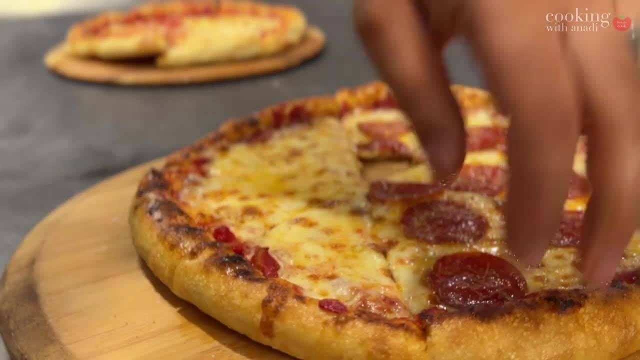 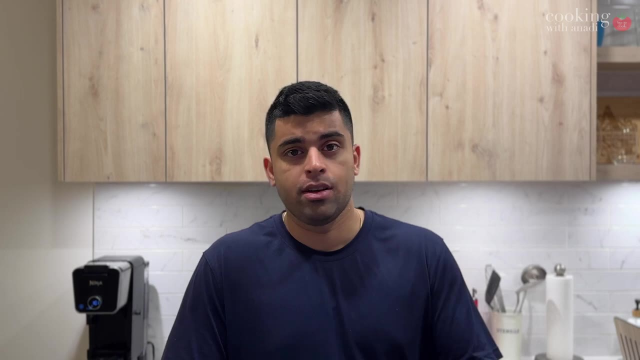 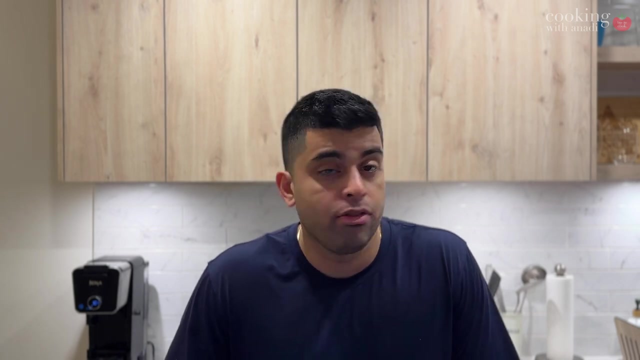 these two types of flour apart when it comes to a Neapolitan pizza- and, mind you, this only applies to the Neapolitan pizza or a Neapolitan pizza- it's not a blanket judgment on all pizza types because, depending on the type, a different flour might be better over the other. let's find out more in this battle of. 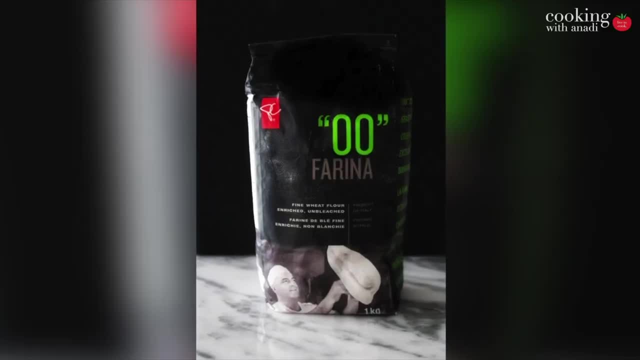 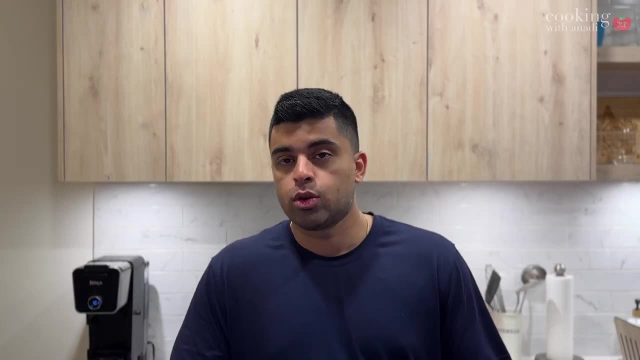 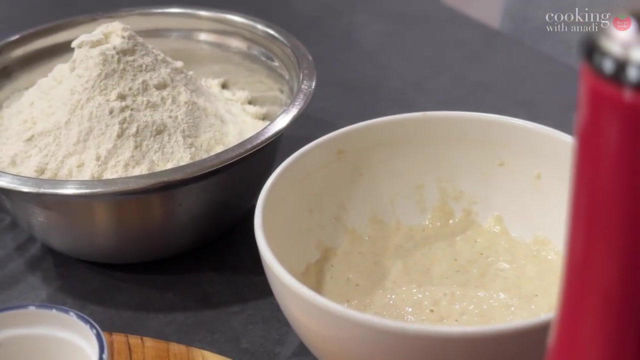 the ingredients. so if you're new here, you've never seen me do a double oh video before. well, this is a grading system that Italy uses to really show how finely ground or milled the flour is. in this case, the double O is the name of the flour, simply referring to the level of the grind of the flour, how fine it is. 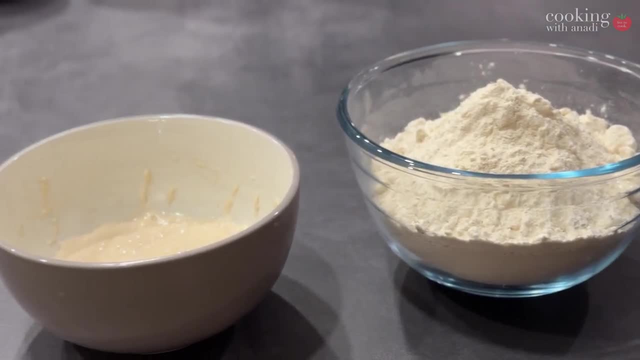 compared to other flours, and double O is the gold standard of flour that's used in Italy and pizzas make. a good pizza with a good quality of pizza and a good quality of pizza is a good pizza with a good quality of pizza and a good quality of pizza and a good 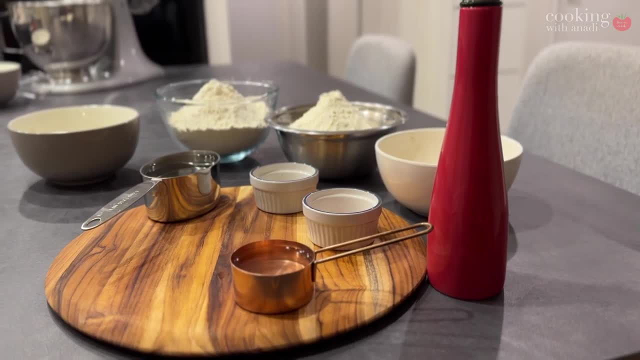 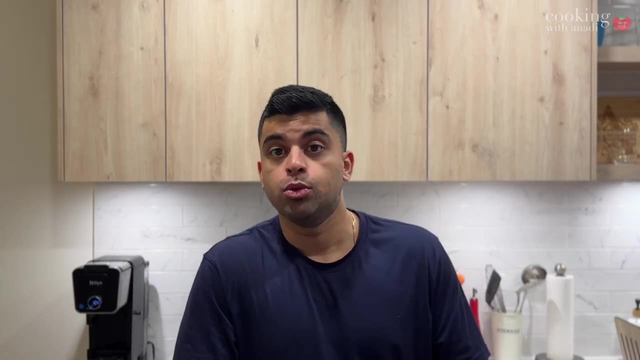 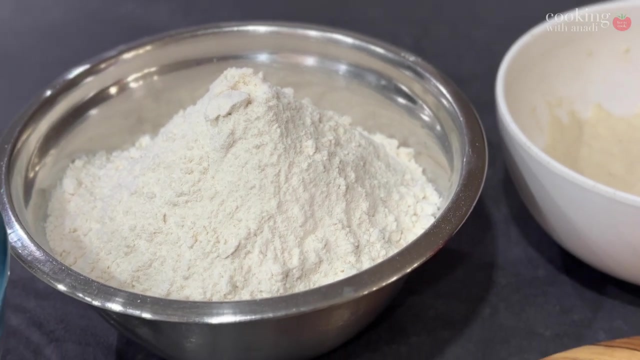 with this flour are usually really fluffy, light and crusty and usually used to make napolitana style pizzas. now, the dough that i'm making today is using a starter, specifically a poolish starter, and while kneading i noticed some key differences between double o and the bread, flour dough and 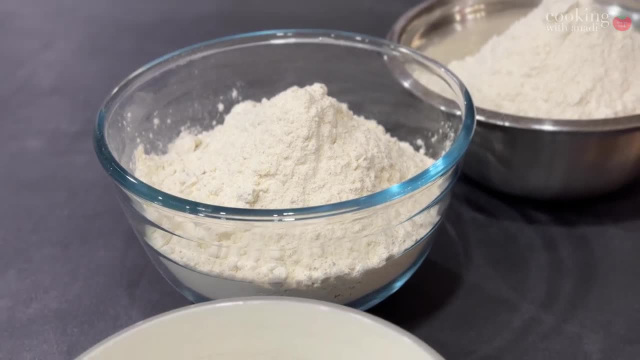 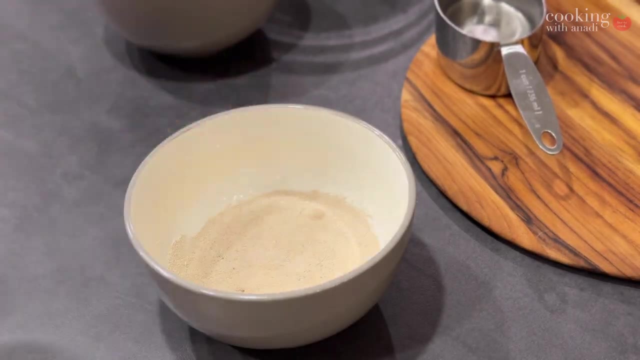 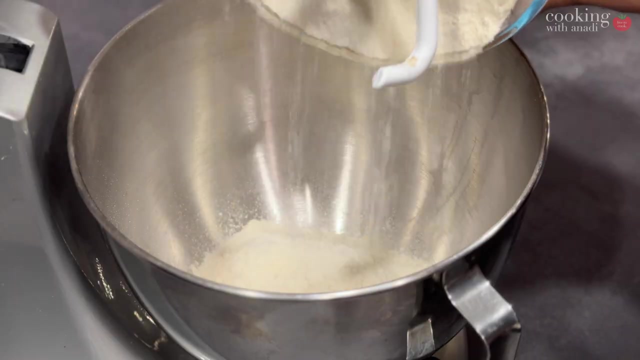 traditionally double o because of the type of flour it is, it's a bit lower protein content than the bread flour, which has much higher levels of protein. was that it was much easier to get a soft um kind of dough with the double o flour, with less knead time when compared to bread flour. 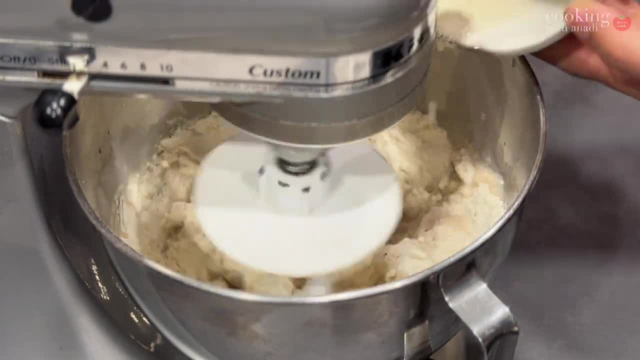 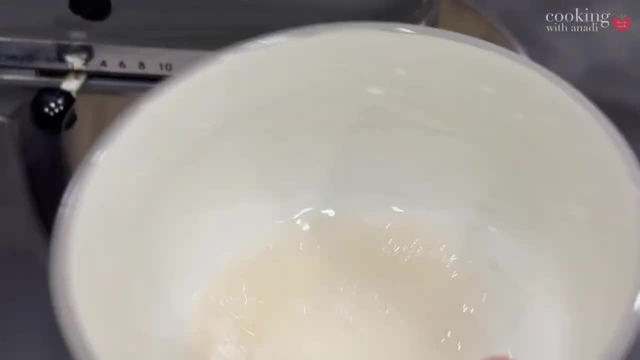 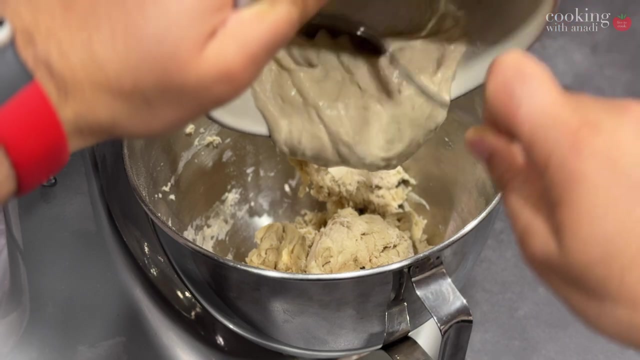 so bread flour has just higher amount of gluten as well, while the double o has a moderate amount of gluten. and to really get that same elasticity, the softness and the smooth dough that you're looking for in a 00 flour for a great Napoletana pizza, You just 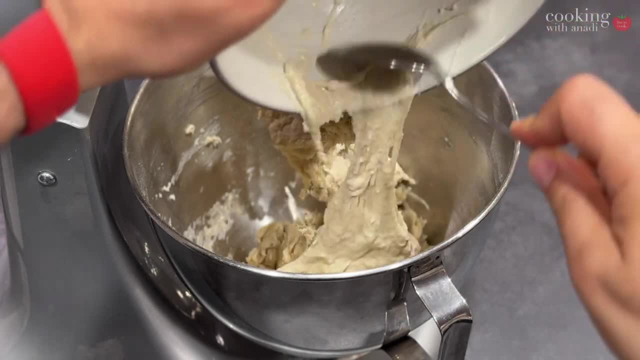 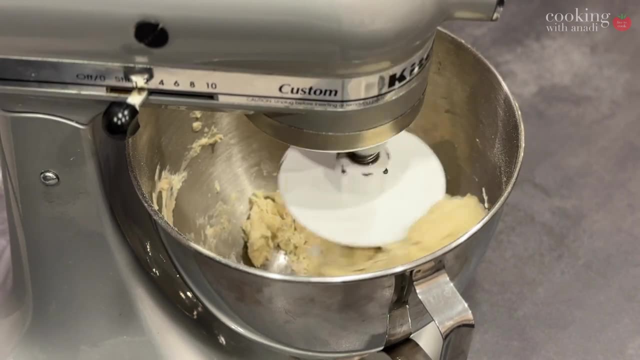 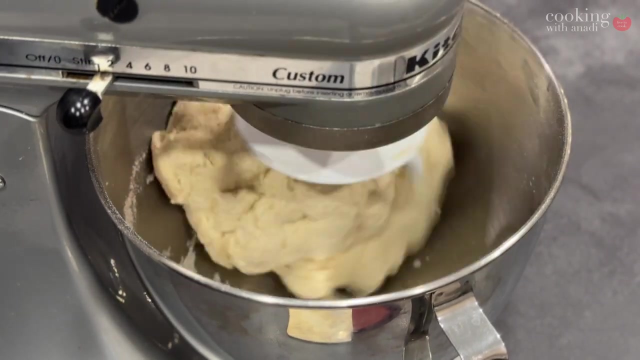 need much more kneading to get that same kind of texture to the bread flour And it really takes a village. I guess in your mind that you're kneading to really see what's happening and then pivot and adjust from there right So that you see how much more hydration it needs. 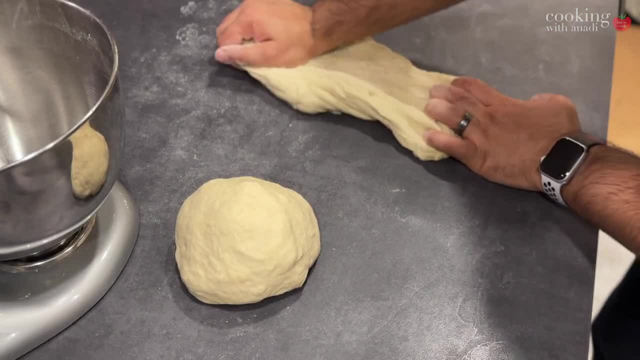 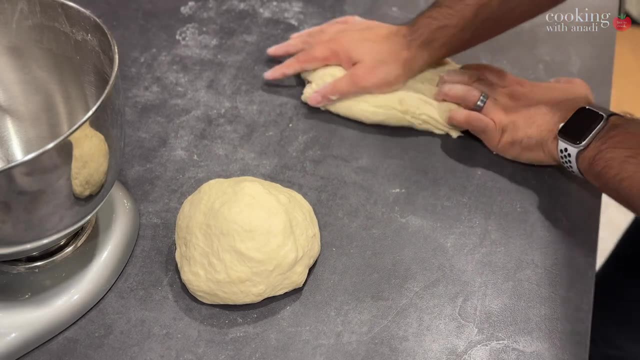 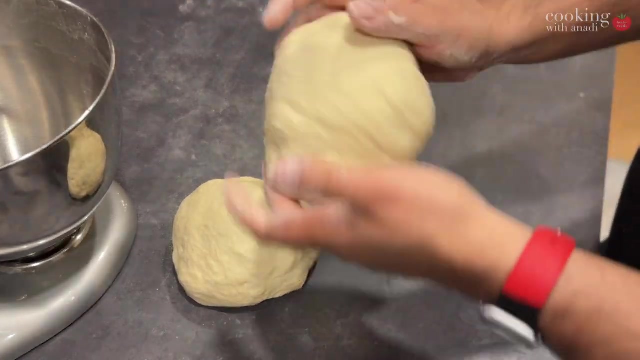 how much more kneading it needs so you can get the same sort of dough. because we want consistent results And because of the extra knead time, one of these pizzas is going to be a little bit chewier, which is not a bad thing, Like, let's say, let's say- naan bread. I love when it's chewy, It just. 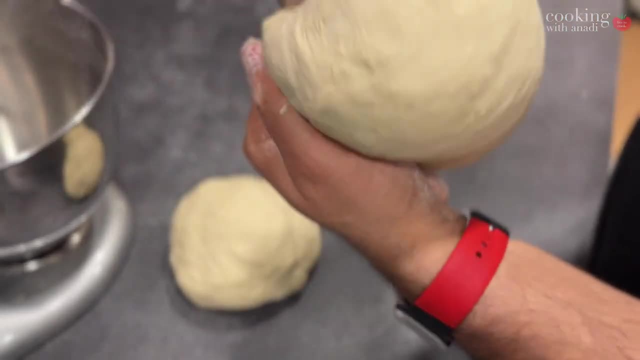 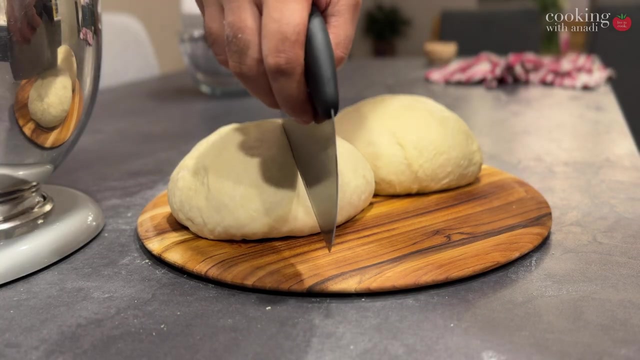 adds so much body to it, And if that's what you like in a pizza, then that's great. But one of these pizzas we just have a more crusty and soft dough And that's just a whole nother type of experience, Anyways. 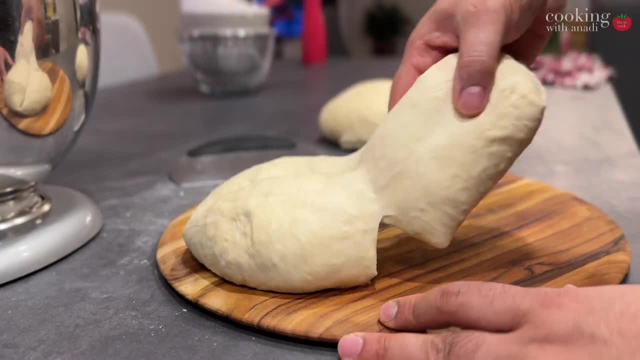 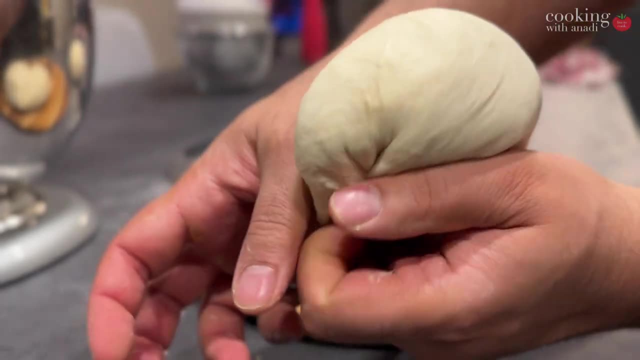 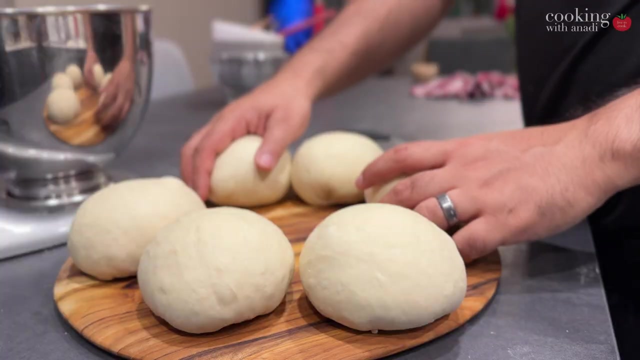 these doughs will ferment for roughly 72 hours. It's going to be more like 65 because the poolish fermented for about 18 hours before being added into the doughs And the doughs will roughly stay in the fridge for about 48 hours. Now, while technically bread flour can be pushed a bit. 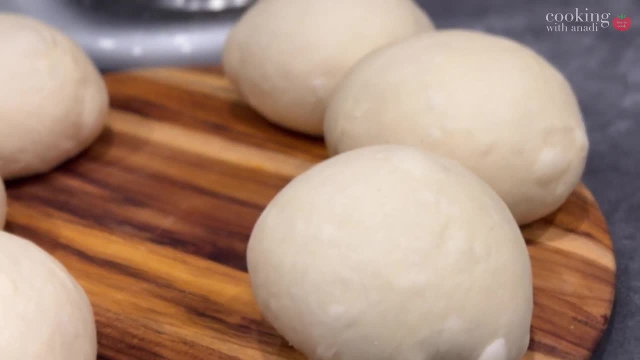 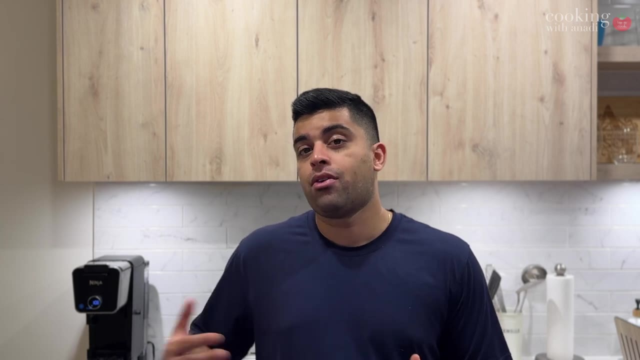 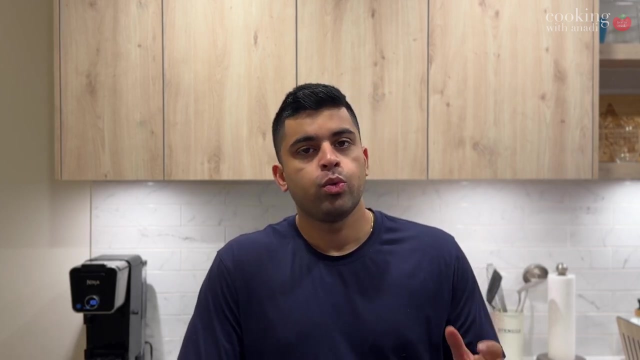 to tolerate much more fermentation. I'm not going to do that Extra work which you can try and experiment to see if you can push it past that 72 hour point, to see if it develops even better texture And if that helps to really relax the gluten, to really give you a softer and elastic. 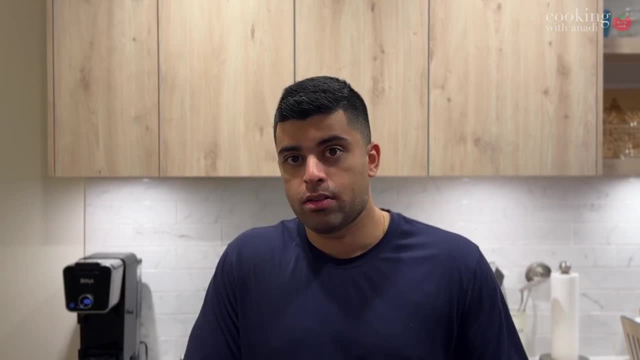 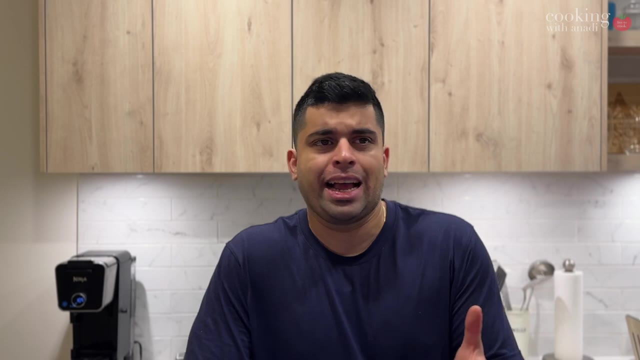 dough, which would be similar to a double O flour dough, which would be similar to a double O flour dough. Now, one big difference that I noticed when it came to the dough was that the dough was not as soft and elastic as it was when it came to baking the pizza. So I guess broiling it. 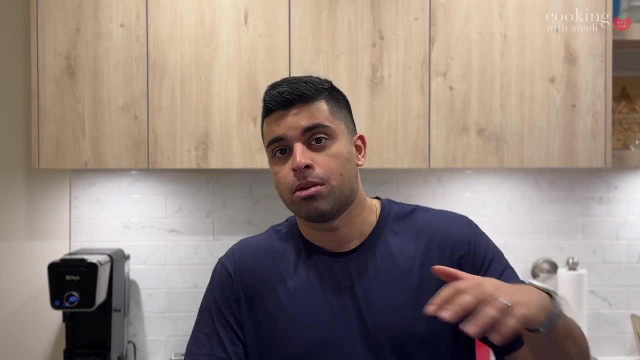 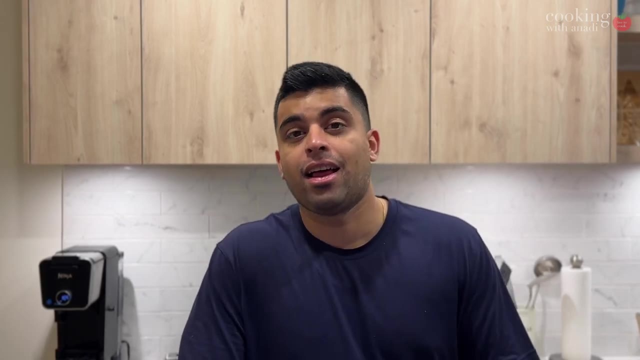 because that's how I make it at home. I don't have a wood fire oven, of course, So I do it under the broiler. Is that the regular flour? Neapolitan pizza did not get great leoparding? Leoparding is. 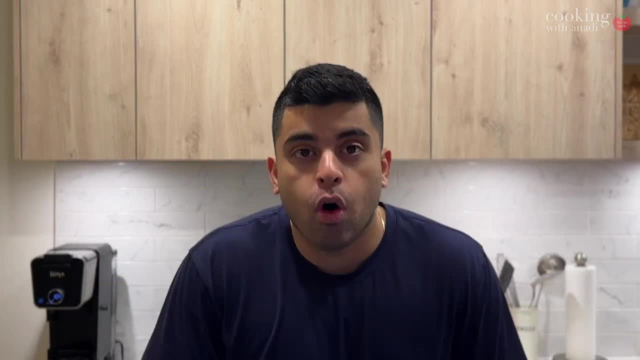 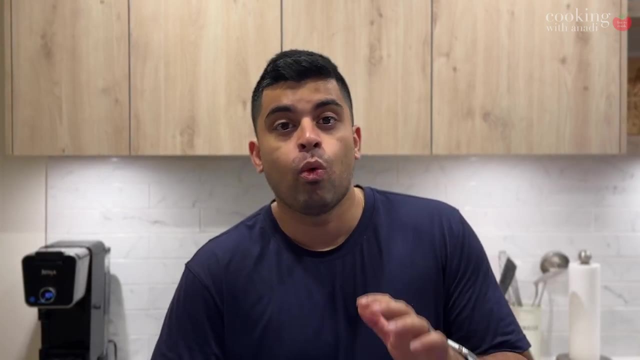 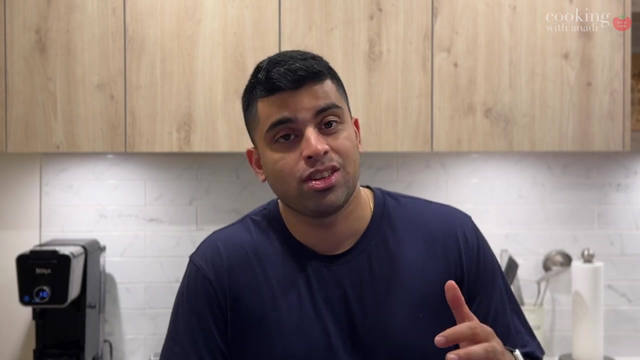 just like the black spot that you get all around dotted on the pizza And it just shows like how the crust is reacting and cooking under high heat. The pizza that had an amazing leoparding and texture and crustiness was the one made with the double. 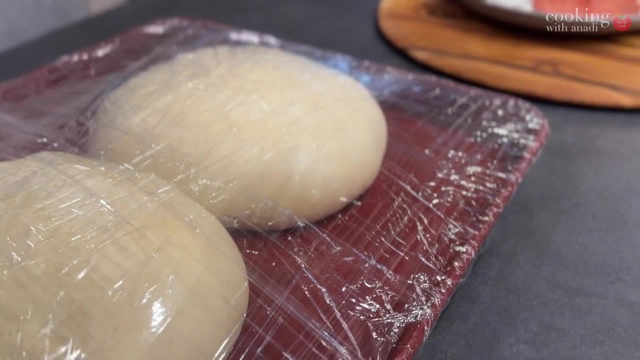 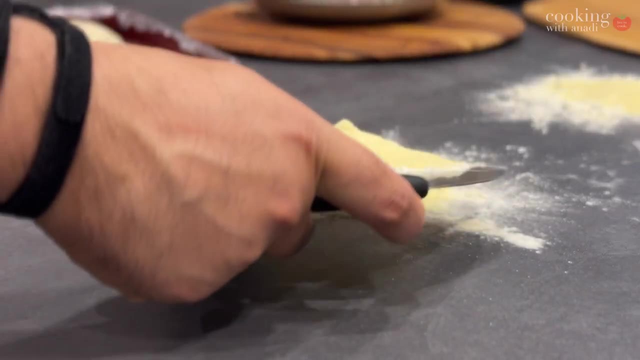 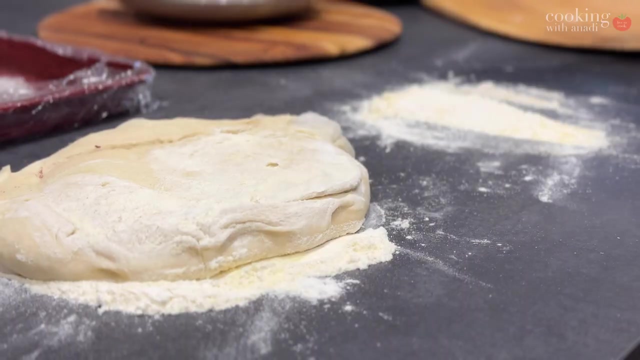 O flour. Well, in this case, check out what happened So you can see they have risen pretty well And I'm going to scoop it out. This mixture down here is made of semolina and flour. It's going to help to kind of scoop it out And you can see how easily both these doughs are being spread. 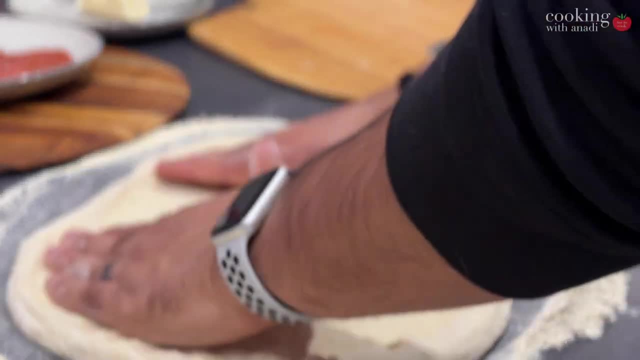 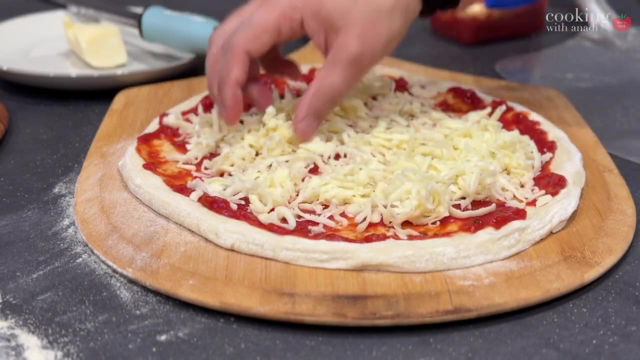 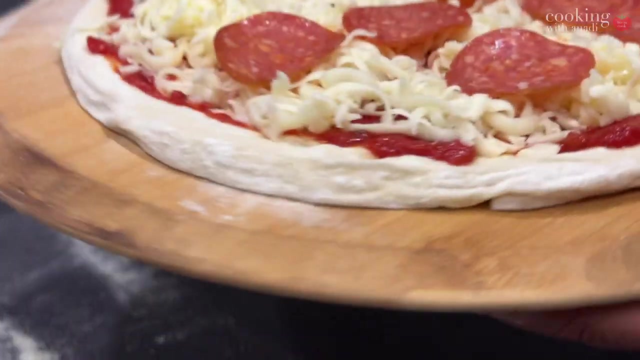 out. It's really minimal effort. if any needed to spread it out. There's some cheese, some homemade sauce, pepperoni on one side and same thing with the other, And we're going to put that under a broiler. Now, mind you, this oven has been heating at 500 Fahrenheit for one hour, which means the 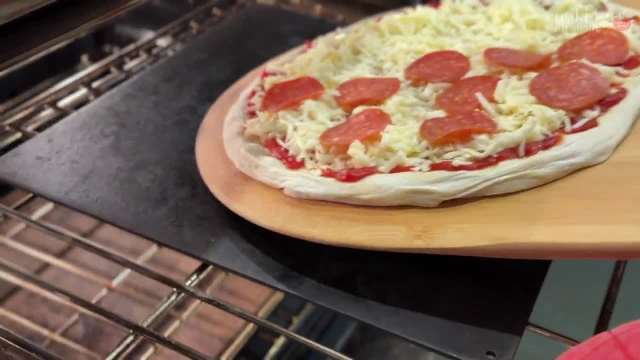 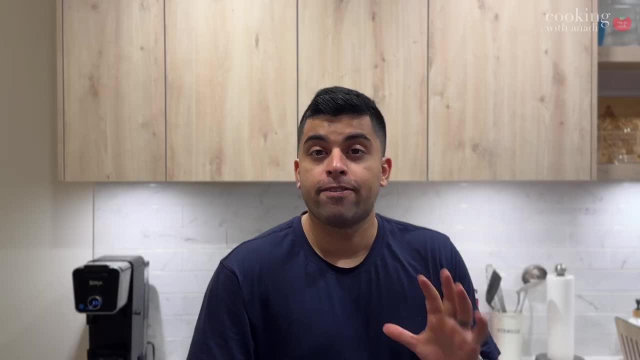 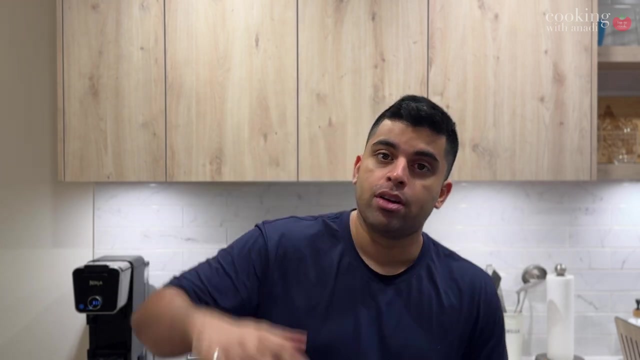 oven got to 500 and it's been heating at 500 for one hour with the stone and the steel, And then the steel has been under the broiler for about five minutes. That bottom is really hot and it's going to go right under that broiler as it starts to cook. And that high, intense heat is what kind. 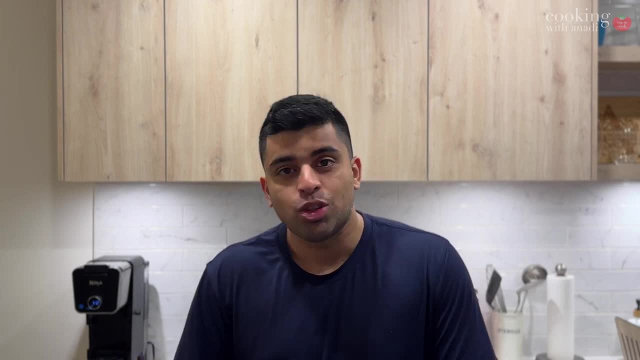 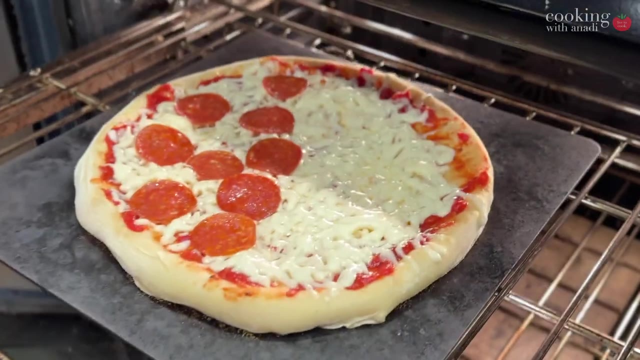 of tries to simulate a wood fired oven that's usually used to make Napolitana-style pizza, except this time it's at home. I turn it once, always after about 30 seconds to 40 seconds. Make sure it's kind of cooking evenly. 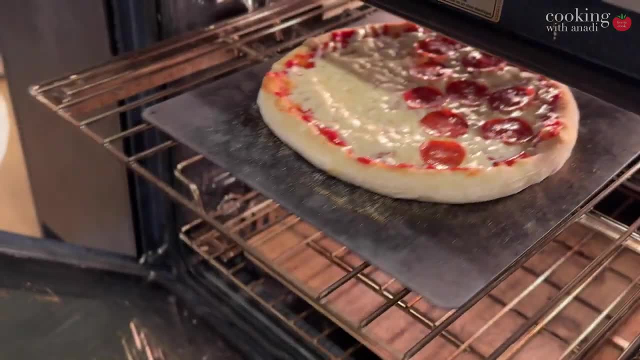 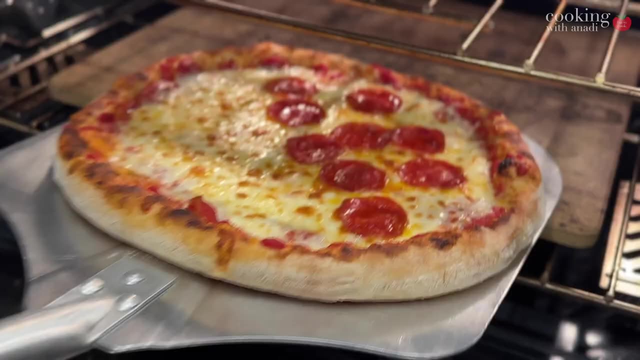 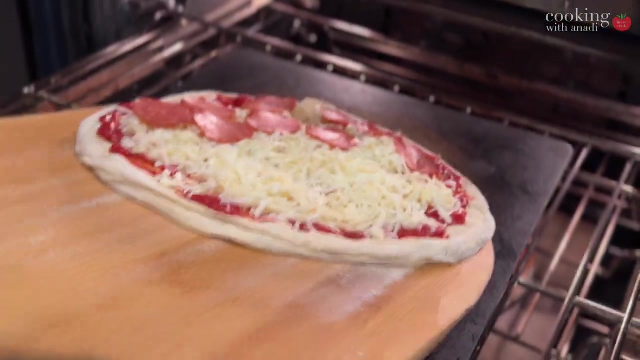 And once I get that browning, that initial color, it goes to the bottom so I can finish cooking the crust. And while that's happening, my second pizza is going in, And I'm sure you all know which one is which. at this point They really look similar. Now leoparding, just to build further, is the. 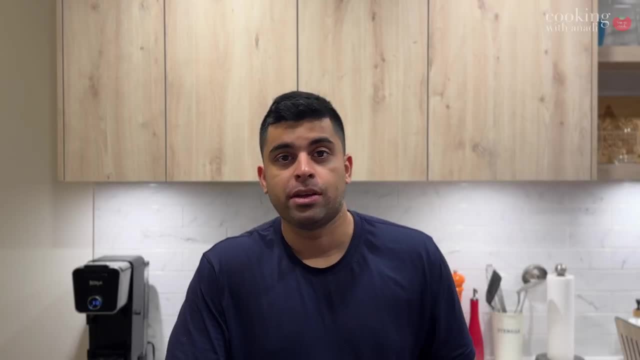 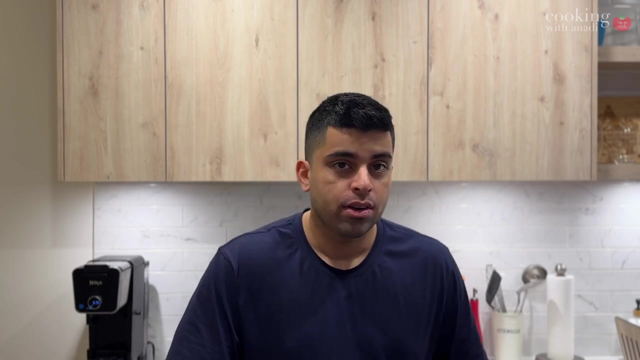 blistering the dark spots that come up on the crust of the pizza when cooked under high heat, And I think both these pizzas have really similar looking- leoparding. I didn't go overboard with it, I didn't let it get too dark. 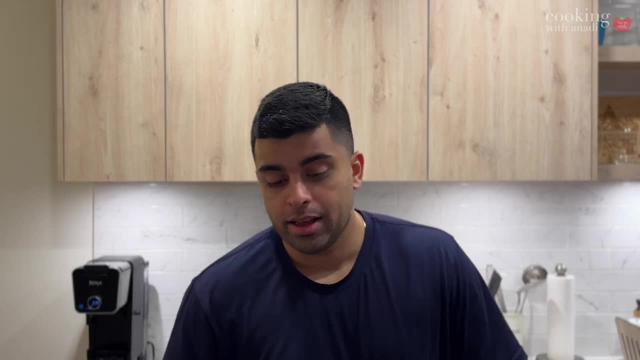 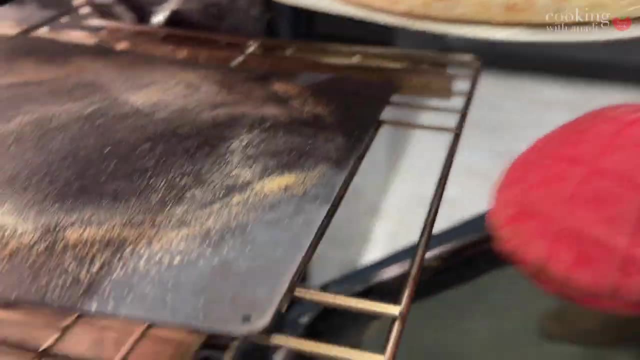 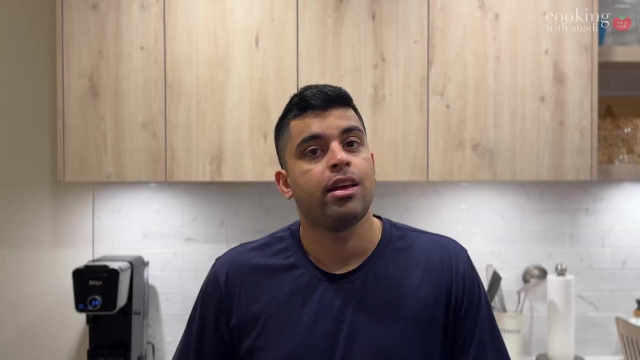 But what we got, the brownness, it's very hard to tell. So it's very hard to tell which one's which still. So what are the differences that I've noticed so far? Well, the bread flour. it took longer to knead to get the same elasticity, softness and all. 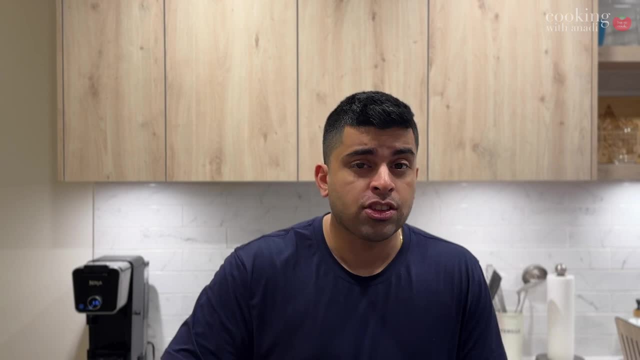 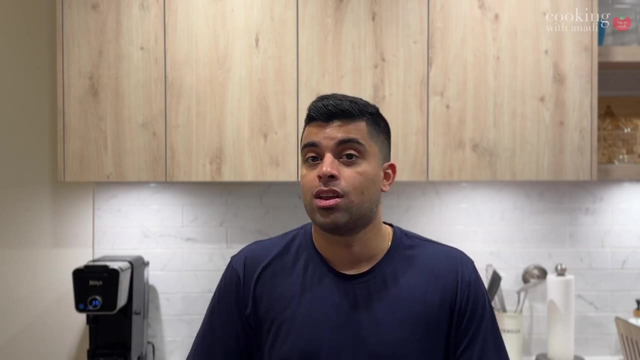 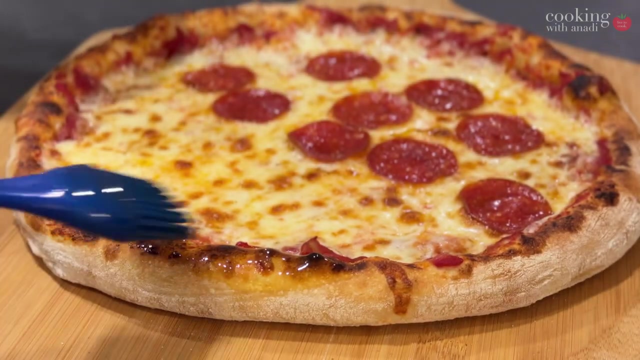 It took a bit longer in the oven to get the same color texture and the leoparding that I'm talking about for the bread flour pizza when compared to the double O flour pizza. But that really is superficial. It's just some time that's extra, Maybe like five minutes max, It's nothing. 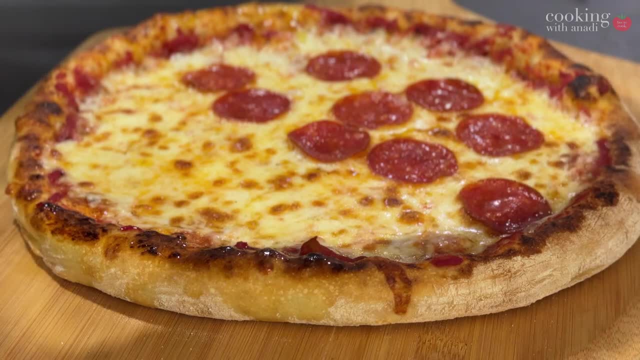 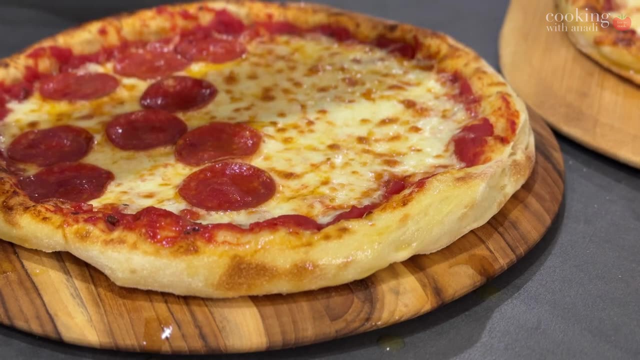 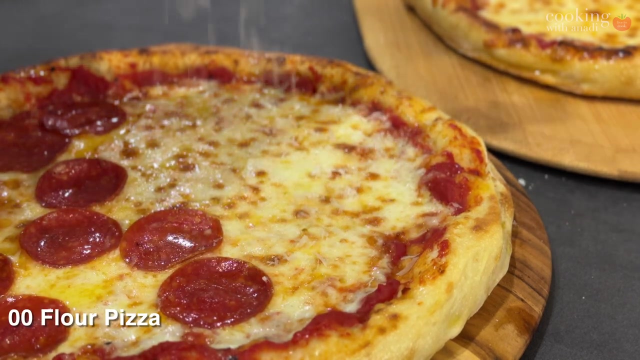 The proof is in the pudding, It's in the eating. So the only way to really tell if there's any proper difference, That's notable, That's worthwhile, is by tasting, And I can tell you which one's which. The pizza that I took out first from the oven was the bread flour pizza, And the pizza that I took out second 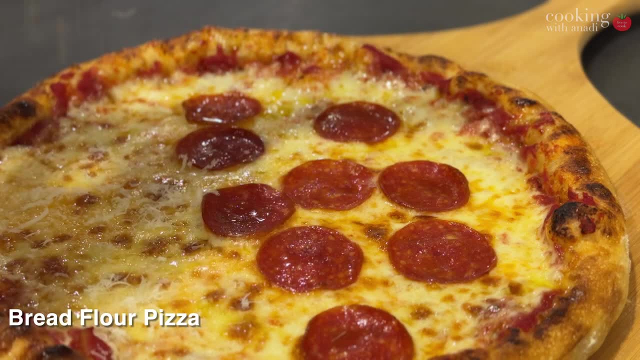 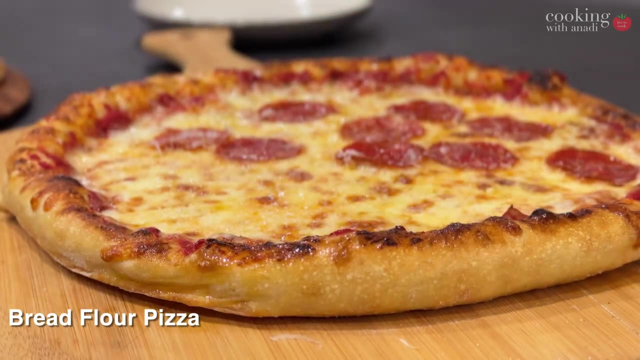 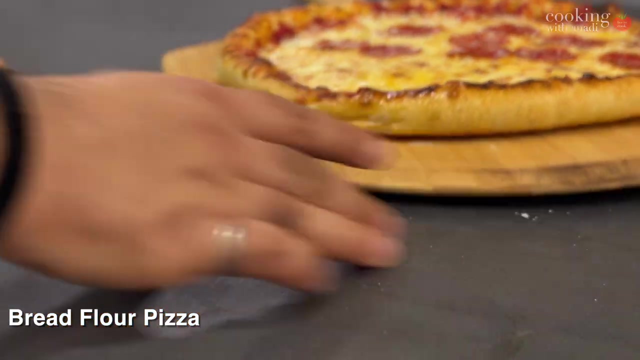 was of course the double O flour pizza. And here's what stood out: The bread flour had a very satisfying chew on the crust. Very satisfying, A nice initial crunch And then nice satisfying chew with the sauce, the cheese, Amazing.